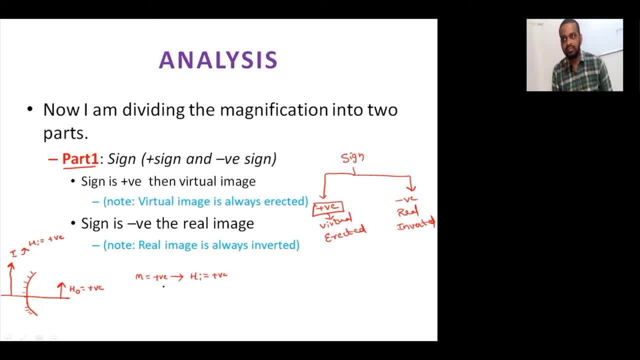 of the height will be positive. so that's why the positive magnification is produced by only a, a, a, a virtual image. and coming to the negative magnification, in order to get the negative magnification definitely, the image should be formed below the principal axis. then only the height of the image is negative. the height of the image is 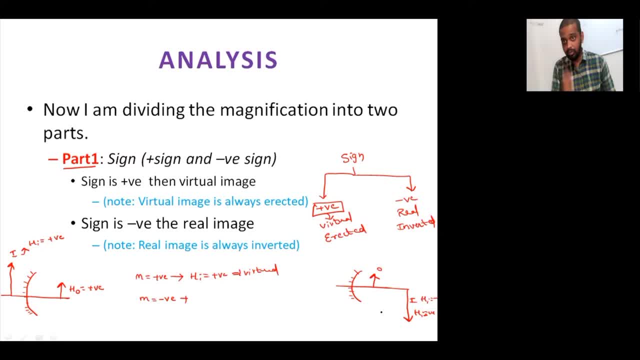 negative. now the height of the image is negative. when height of the image is negative, then we will get the image as inverted image, which will be from outside the mirror and it also considered as a real image. only the real image will form outside the mirror, which is inverted. so, in order, 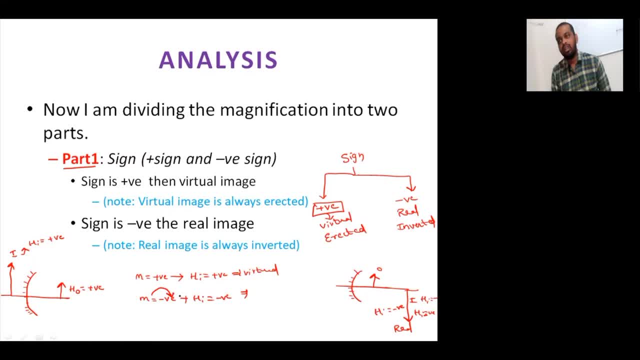 to get the magnitude magnification as negative we have the only possibility to have. height of the image is negative. height of the image is negative, then it will be from outside. the mirror which is inverted lies below the principal axis, so it will be the real image and also i. 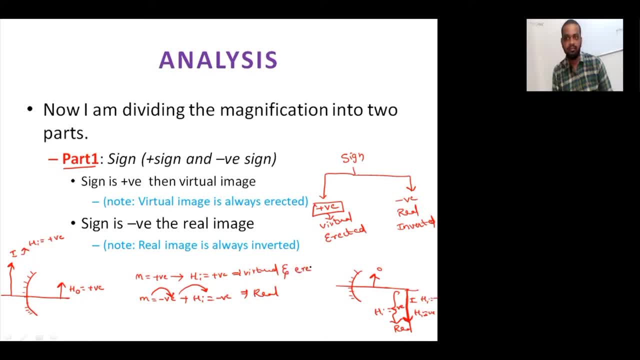 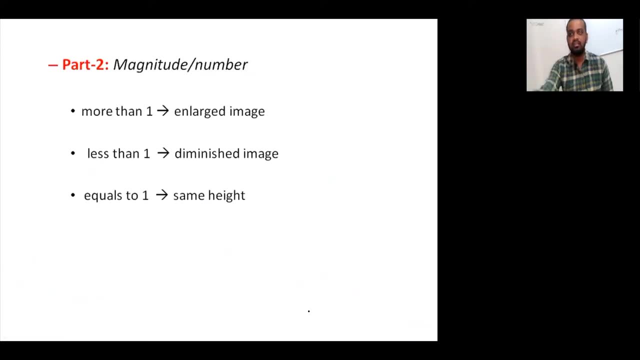 clear that virtual image is always erected and the real image is always inverted. so if the magnitude magnification is positive, then it will be the virtual erected image. if the magnification is negative, then it will be the real inverted image. now we will discuss about the part two. 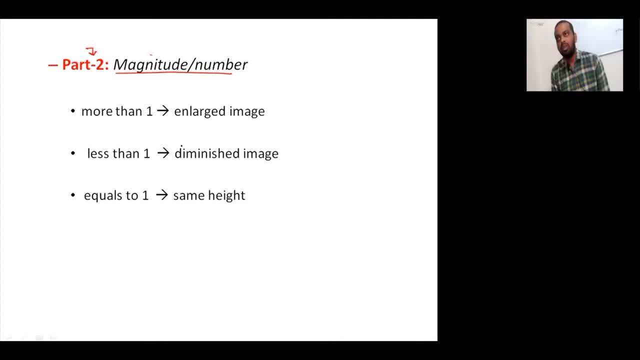 so part two is nothing but the number, only number, nothing but magnitude. then the number is more than one, nothing but magnitude is more than one. then what will happen? height of the image divided by height of the object, magnitude will be more than one. then height of the image is more than height of the object, which leads to form the enlarged image. 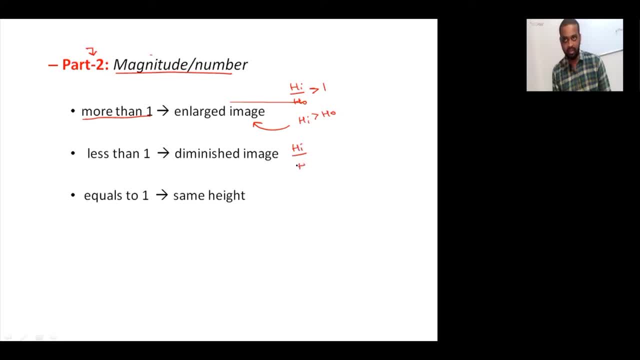 if it will be less than one magnitude is less than one. h i by h pro will be less than one magnitude. Magnitude is nothing but modulus. Here we don't consider negative sign. Remember this thing. Then h i is less than h o, which leads to form a diminished image. 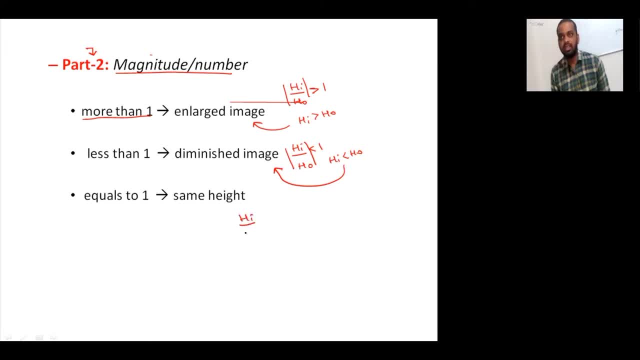 If it will be equal to 1, then h i by h o mod of h i by h o is equal to 1.. So if you put it in the mod after removing the mod, if h i by h o is negative. 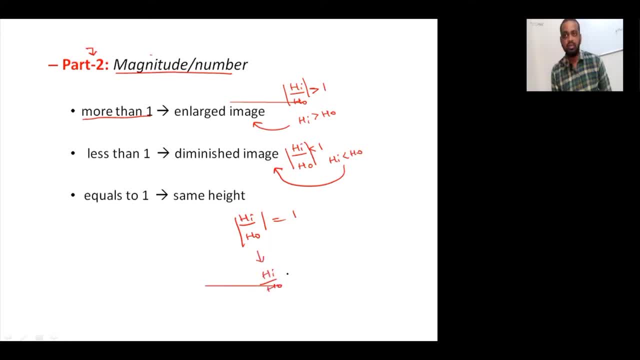 then you should consider it as only the positive value h i by h o is equal to 1, then h i is equal to h? o, which leads to form same-heighted image. Now we will discuss this concept with one example. 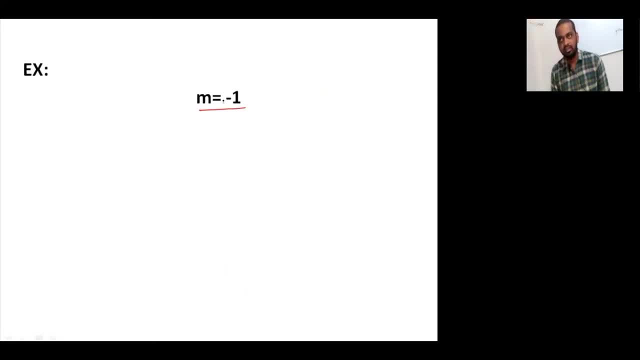 Now I have taken the magnification as minus 1.. So as of part 1,, part 1 is sign, which is negative sign, And the part 2 is the number. nothing but magnitude, Only number. you should take children. 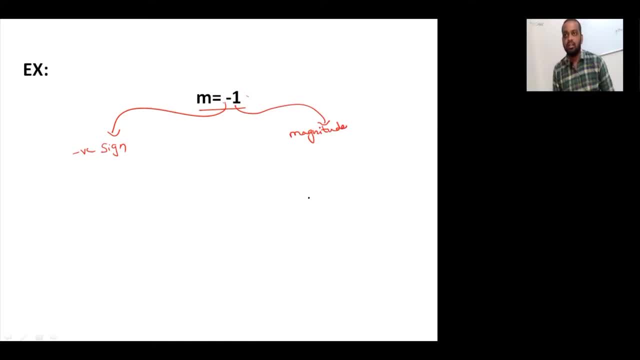 Don't take minus 1. It will be leads to the wrong option, wrong answer you will get. Magnitude is only 1. you should take, only number you should take. You should ignore the sign. So the negative sign will indicate it will be the real image. 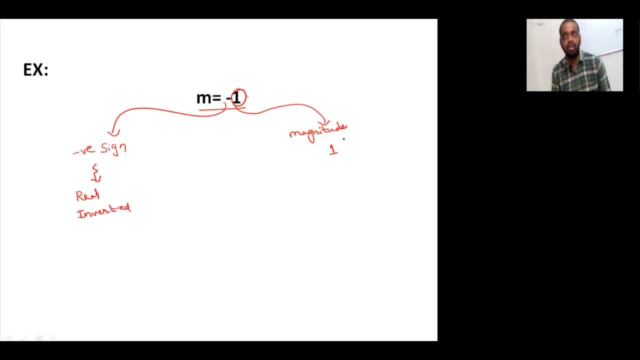 Real image is always inverted And the only number is 1.. So the magnitude of the magnification is 1, which is nothing but h. i by h o is equal to 1.. Now you will have. Height of the image is equal to height of the object. nothing but same size. 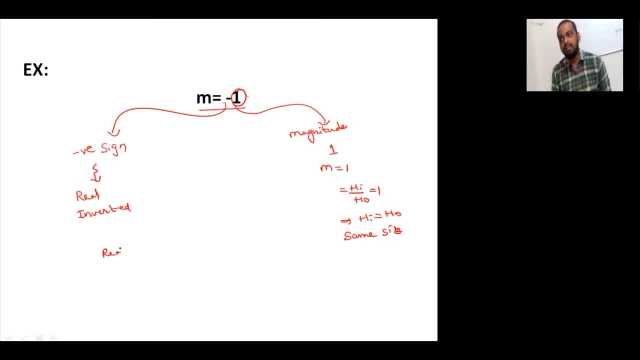 Now combine all the image characteristics- real, inverted and same-sized image- we got: Same-sized image is formed. So we have the only possibility to get this kind of magnification. when you place the object on C, You will get the image also on C. 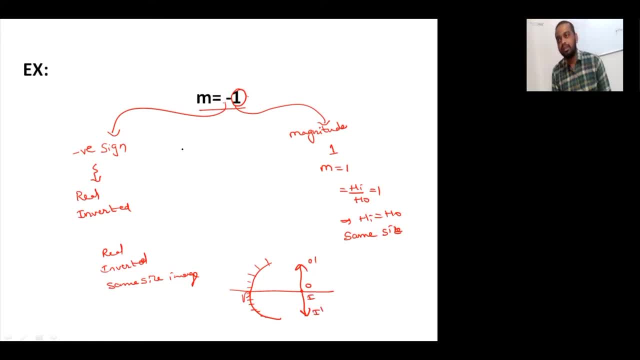 o dash is the object, i dash is the image. So So o dash is the object, i dash is the image. Here it is a concave mirror. Will you guess what is the position? Concave mirror on C is the position of the object. 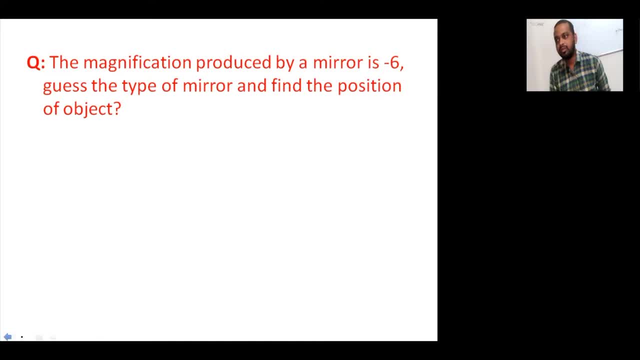 Now we will solve one more question: The magnitude, the magnification produced by a mirror is minus 6.. Guess the type of mirror and find the position of the object. Now the magnification mentioned in the question is minus 6.. 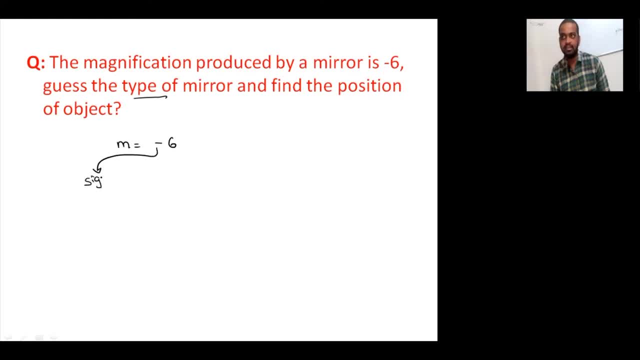 So the So part one is sign. Sign is negative sign. So negative sign leads to form a real inverted image, Real inverted image And the only number that is magnitude. Magnitude is 6, which is more than 1, means height of the image divided by height of the object is more than 1.. 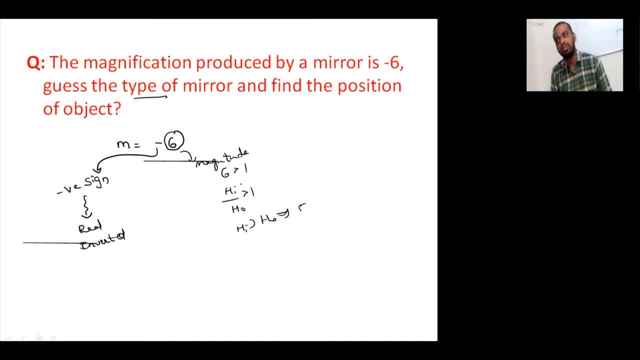 So height of the image is more than height of the object, which leads to form enlarged image. So after combining all the image characteristics, you'll get real, inverted, enlarged image. When will you get real, inverted, enlarged image? When you place the object between focus and center of curvature. then you will get the image real, inverted, enlarged image. 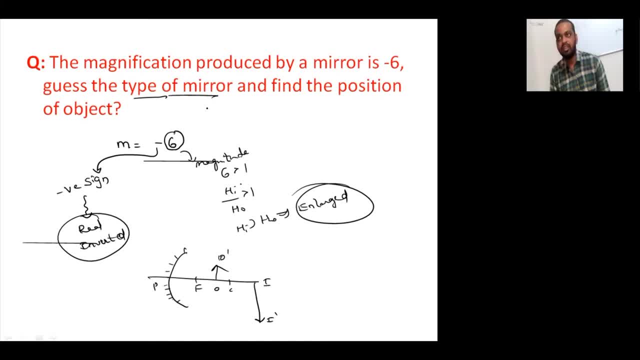 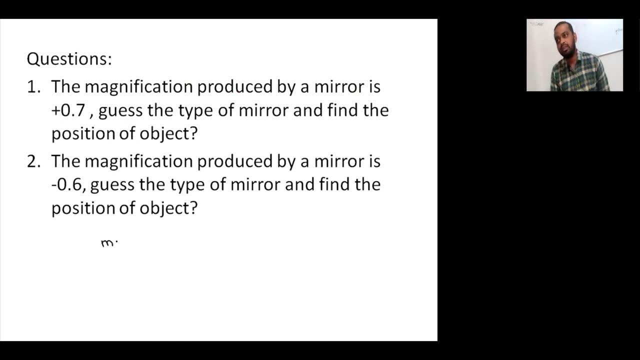 So answer for this question is: the type of the mirror. is concave mirror Concave mirror? And the position of the object is between F and c. now we will discuss some more mc, some more questions. the magnitude produced by the mirror is plus 0.7 in the question number one and in question number two the magnification produced. 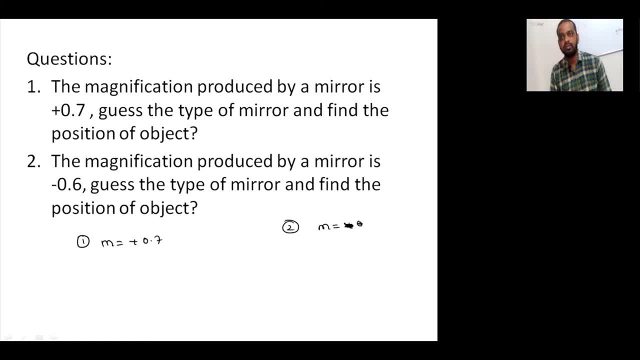 by the mirror is plus 0 minus 0.6, minus 0.6 minus 0.6. first we will solve question number one. so the magnification is positive, so it is virtual image. virtual image is always erected and the number is 0.7. only number is 0.7, so it is less than one, so it is a diminished image. 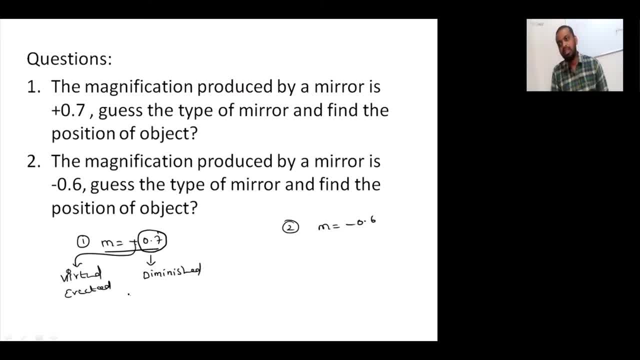 so virtual, erected, diminished image is formed by a convex mirror. and here you should make one important note: virtual, erected, enlarged image will be formed by the concave mirror when we place the object on the mirror. so it is less than one. so it is less than one, so it is less than one. 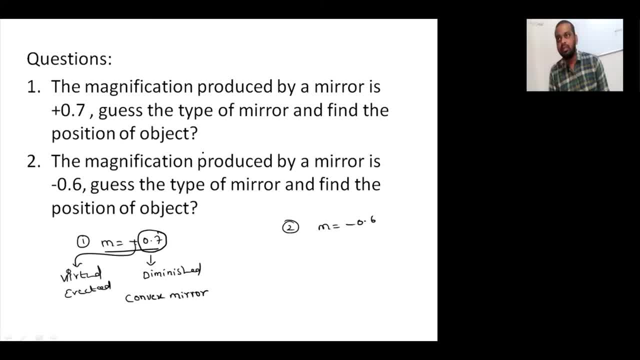 object between pole and focus. so this is the answer for the question. number one is the mirror is convex mirror and anywhere in front of the mirror. if you have any doubts of ray diagrams, you should go through the ray diagrams which i explained to you in the previous videos. now the 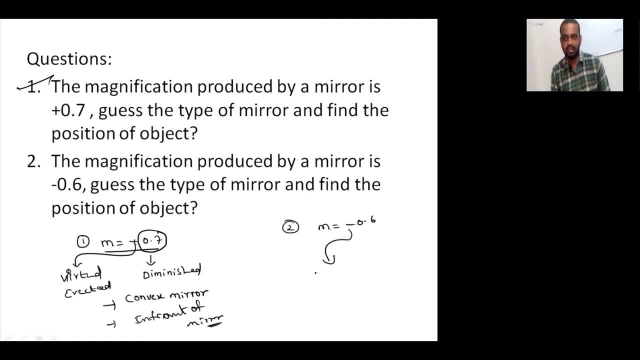 magnification is minus 0.6. minus sign is representing it is the real image. real image is always inverted and the magnitude of the magnification is 0.6, which is less than 1, so it is a diminished image. so real, inverted, diminished image is formed by a concave mirror. 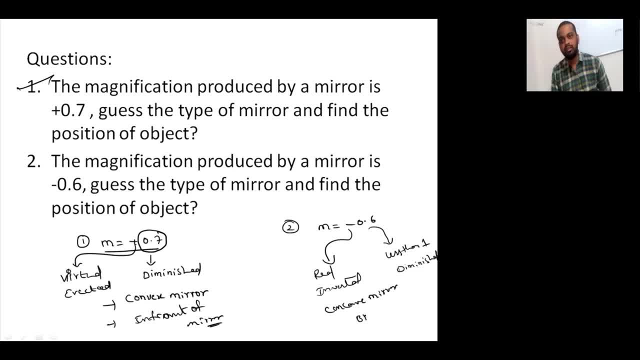 by a concave mirror. when you place the object between- sorry, not between- b on c, when you place the object beyond c, then you will get the real inverted, diminished image and the image is formed between f and c and one in some more mcqs we will discuss contour. mirror produces dash. 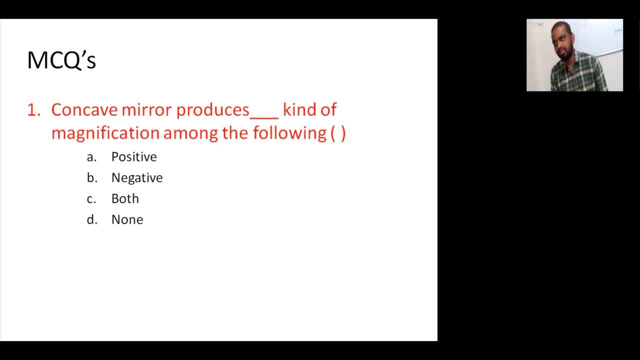 kind of magnification. among the following options here, given as positive, negative, both, none. a contour mirror will form both real and inverted image. for real image the magnitude is negative, for the virtual image the magnitude real, inverted. sorry, a contour mirror will produce real and virtual images. virtual and real images will form a real image is always inverted. 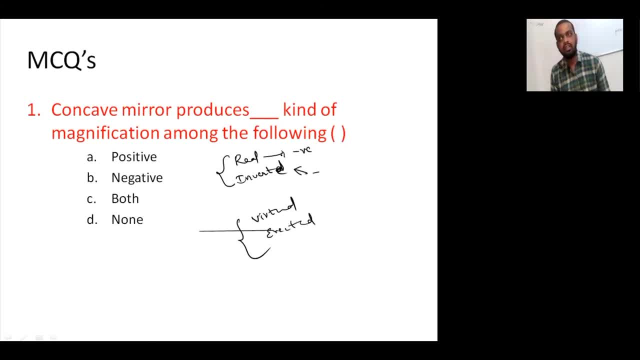 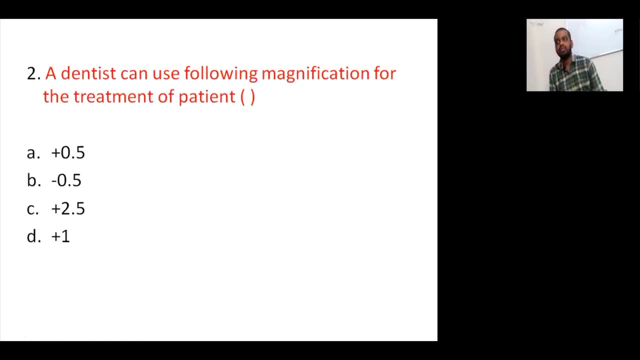 and the virtual image is always erected. for the real image the magnitude is magnification is negative. for the virtual image the magnification is positive. so both possibilities are there. so option c is the correct option. coming to the next mcq, a dentist can use following magnitude: 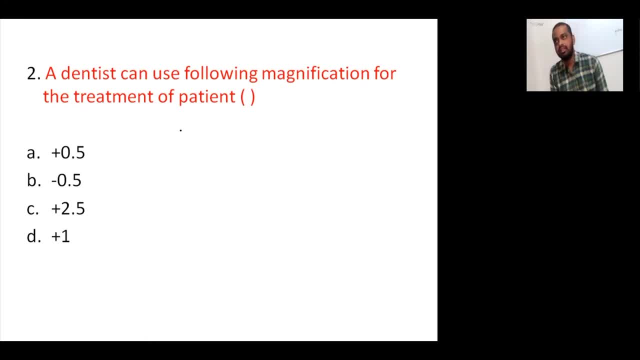 magnification for the treatment of the patient. see, look at here a dentist. use only concave mirror. why? because a concave mirror will produce virtual, erected, enlarged image. he will adjust the teeth between pole and focus so that the image of the teeth form inside the mirror, which is virtual, erected enlarged image, so that 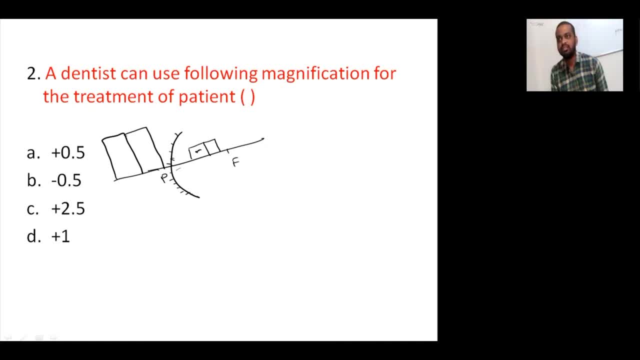 is very simple to identify which part is not good on the teeth clear. so here the teeth image is enlarged and the image is virtual. always it is erected and enlarged. so this kind of magnification we need to find out. for virtual image the magnification is positive. for enlarged image the number. magnitude of the number is: 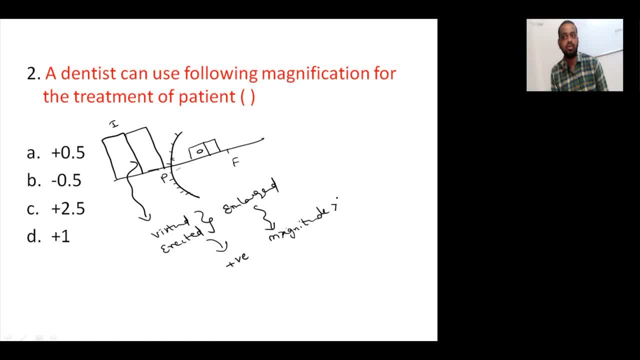 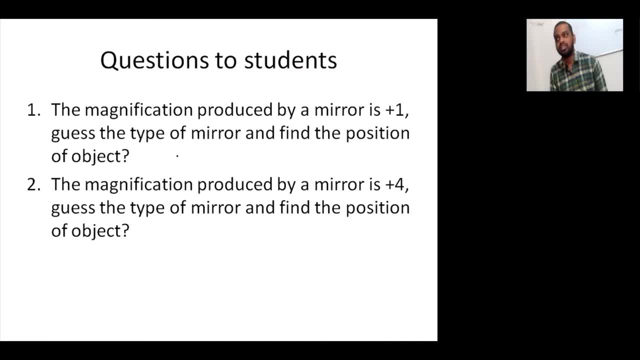 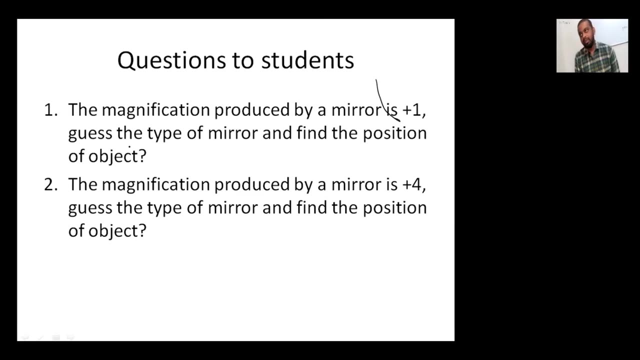 more than one magnitude is more than one. so we have the option c here and some more questions to you. if you have any doubts, please comment below. i will give replay. the magnification produced by a mirror is plus 1. gets the type of mirror and find the position.